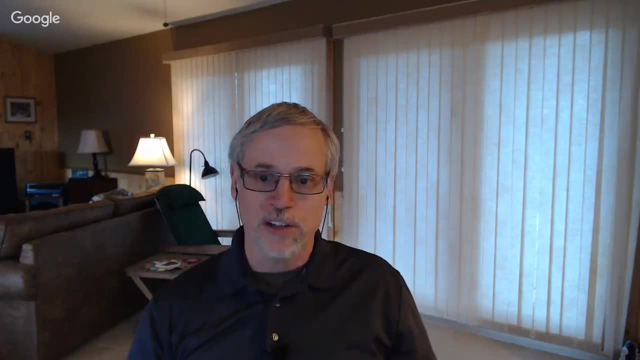 And we'll talk about the MADDPG algorithm itself and then discuss some of those applications, of some of those test environments and how this algorithm fares compared to traditional DDPG algorithm. So with that introduction, let me pull up the slides. So this is the 13th webinar for the DDPG. 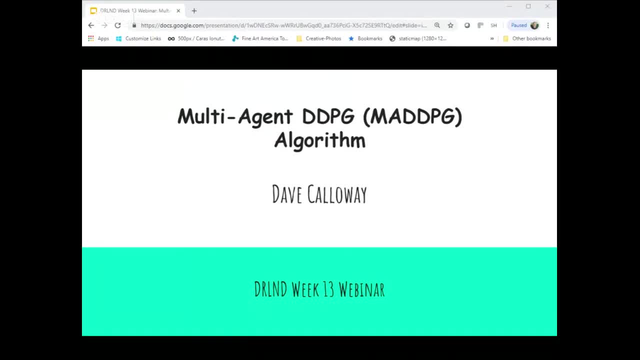 I'm a deep reinforcement learning nanodegree at Udacity and we've covered quite a few topics up to this point, And this is kind of a more advanced algorithm. It builds on one of the actor-critic algorithms we talked about last week, the week before deep deterministic policy gradients. 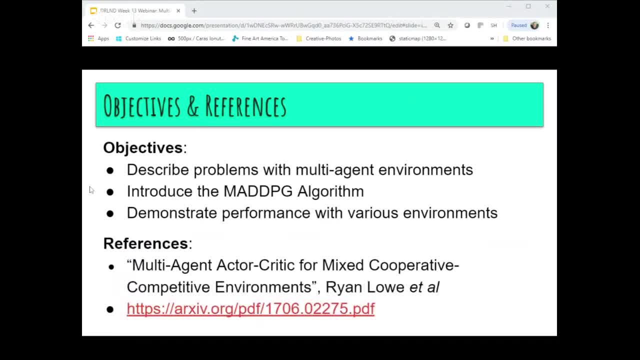 So actually to start with, I probably should reference the references. This is a review of a paper, a research paper by Ryan Lowe and others. It's a title Multi-agent Actor-Critic for Mixed Cooperative Competitive Environments, And I have the archive link there. 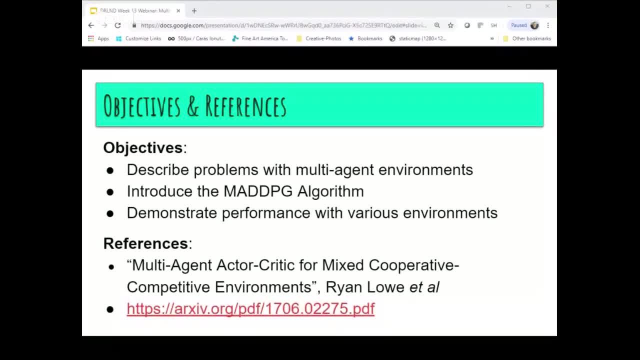 It's an interesting paper. I really would encourage you to pull the paper up and take a look at it on your own. This is just sort of introduction to that paper, And there's certainly more detail in the paper itself that I won't cover this evening, but I'll try to touch on the main topics. 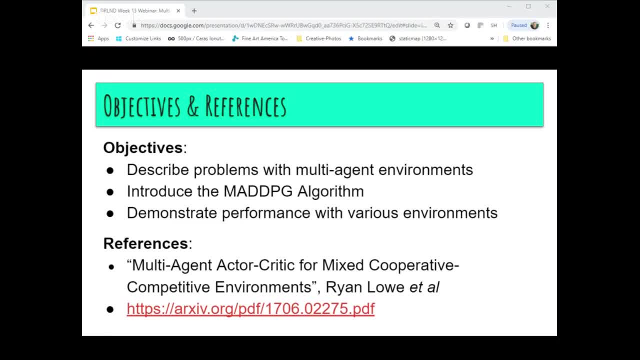 So the objectives today primarily really describe the problems that traditional algorithms might have when there's multiple agents either cooperating or competing with one another in a single environment, And then introduced this multi-agent DDPG algorithm that is the main topic of the discussion this evening. 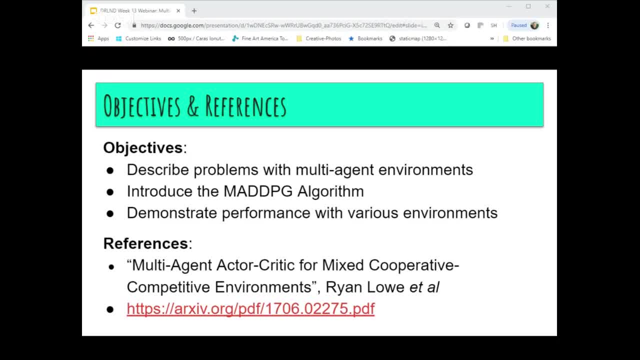 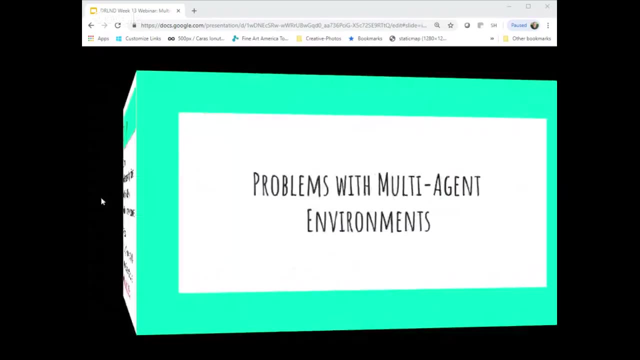 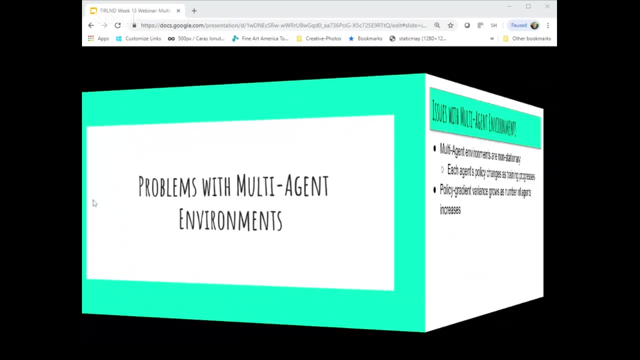 And then at the end kind of compare the performance of this new MA DDPG algorithm to the traditional DDPG algorithm and see how this extension actually does a better job in these types of environments. So to begin with, there's a couple of problems with multi-agent environments. 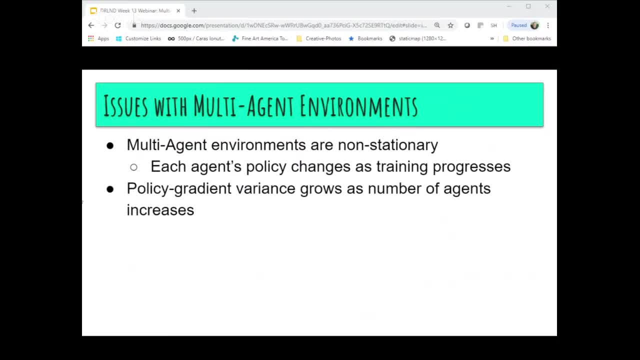 So let's talk about those. The first one really is a situation that complicates learning, and it's when environments are non-stationary. So typically in the environments we've talked about in the past, the environment is pretty much the same from episode to episode. 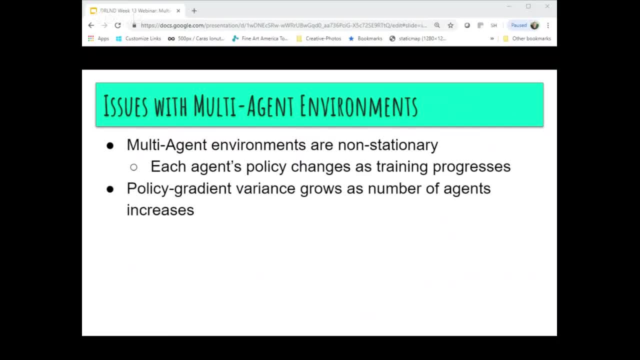 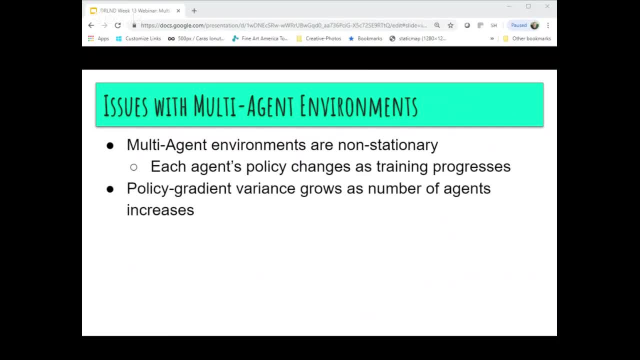 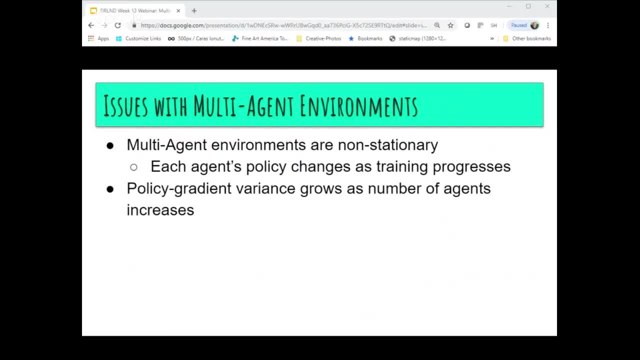 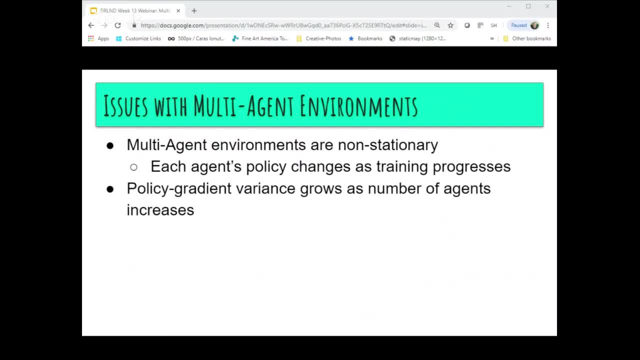 And the agent can run multiple episodes and kind of see the same thing. And the agent can run multiple episodes and kind of see the same thing. And the agent can run multiple episodes and kind of see the same thing. ability to really understand the environment and know what action would be best in a particular 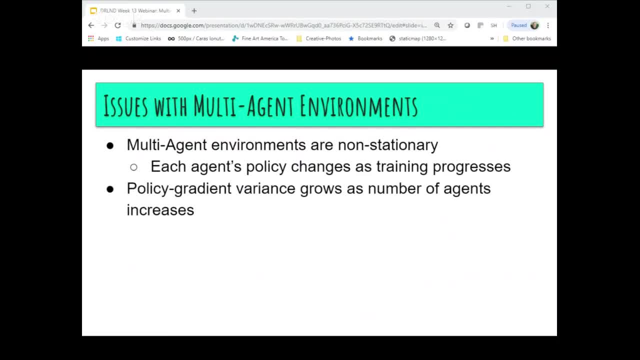 situation And the actions of the other agents might change what action is appropriate, even with the same observations. The second problem is that as you have more and more agents, the gradients increase in variance and that additional variance really complicates the policy gradient kind of techniques and it becomes more difficult to learn and learning. 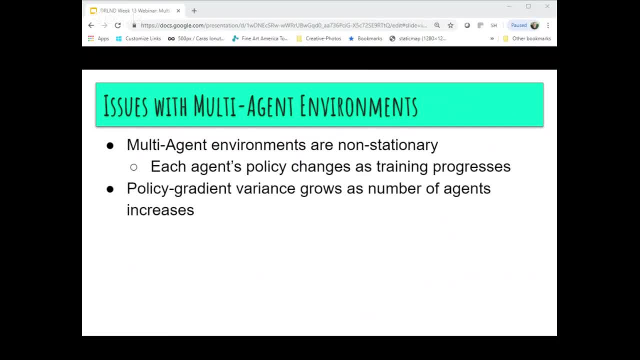 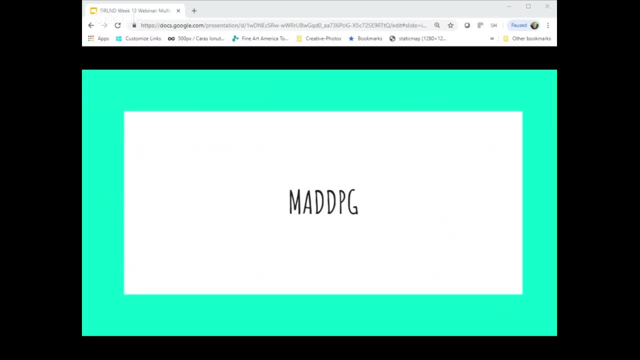 is slower and maybe becomes unstable. So now let's talk about this MADDPG algorithm and see how it addresses some of those concerns and how it works to solve some of these problems and improve learning in an agent's learning of the environment. So it's really a 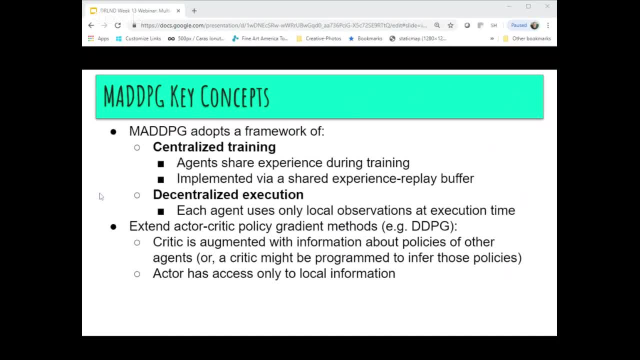 real simple concept, and it's based on a framework where the agent has two key things: One is centralized training and the other is decentralized execution. So what do we mean by those two things? Well, centralized training means that the agent that's learning about the environment. 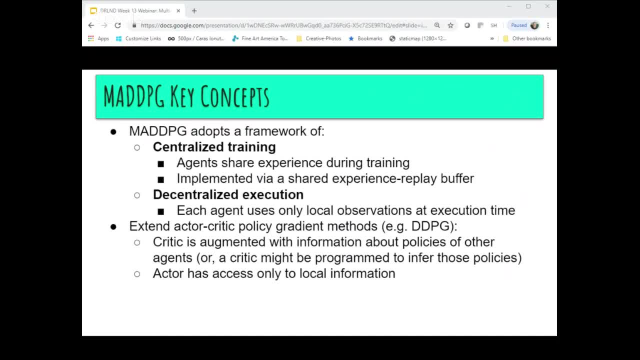 can actually share experience from all the other agents that are interacting in the environment, and all those different agents experiences can be put into a single shared experience replay buffer and then the first agent has access to all that experience and can use that to this kind of helps with the non-stationarity idea here, by having knowledge of everything that's. 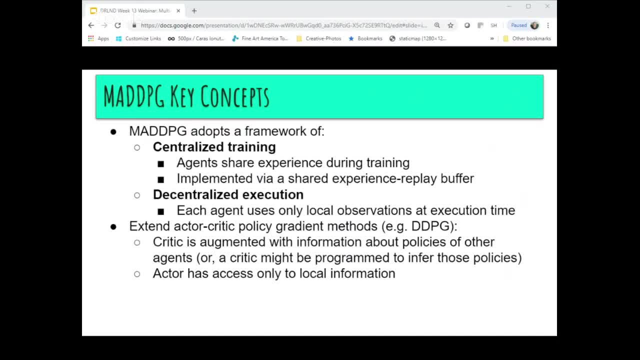 going on with all the other agents. It kind of helps the first agent understand the environment better and be able to learn better actions to take in different situations. You might think that that would work in execution also, but the problem there is that if you actually enforce that in execution, it means that every agent basically has to be omniscient and 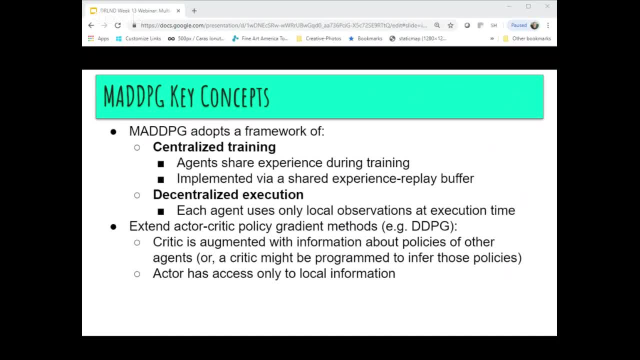 know about every other action taking place in all the other agents and that kind of could complicate execution environments. So the goal is that, even though you might take advantage of all that extra information during training, you don't want to, you do not want to have to rely on all that data. 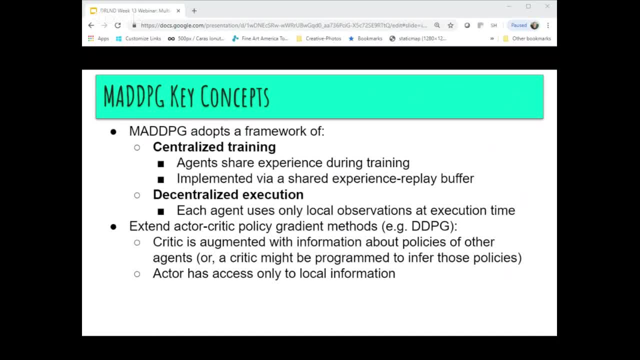 during execution, and the agent ought to be able to. the trained agent ought to be able to take what it sees in the environment and, based on his training, take appropriate actions in that environment. So again, centralized training, but then decentralized execution. So how's this accomplished Really? the author started with a classic algorithm for actor. 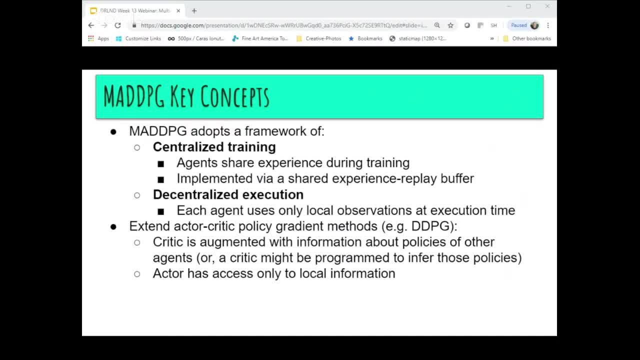 critic type of environment, of training environments, and that's the DDPG algorithm One. you should be very familiar with the final two projects in this course. The first one is the DDPG algorithm. It's not required, but most students end up using DDPG as the as the algorithm that's. 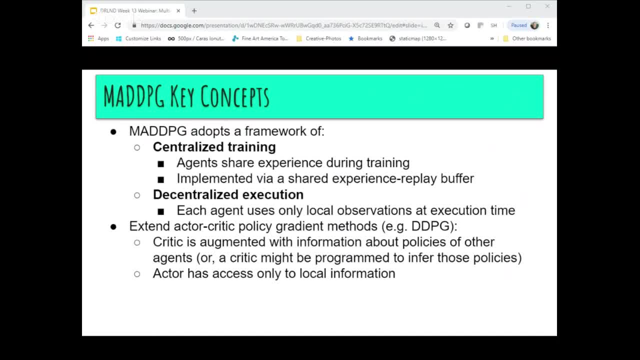 implemented to solve those two environments and in fact, in the final project, MADDPG, the multi-agent version of that is the one that most students actually try and find success using, so it's it's useful to understand this algorithm and it's a very simple extension to DDPG. 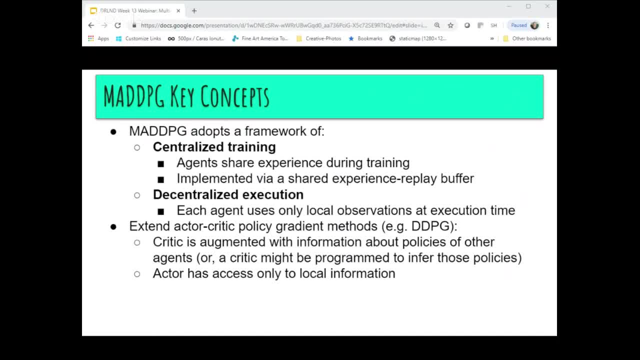 The simple answer is that the critic part of the DDPG algorithm is not required. So if you're not familiar with that, you can just go back to the DDPG version and then try and solve those two environments algorithm is augmented to take information about the policies of other agents. this can be, you know. 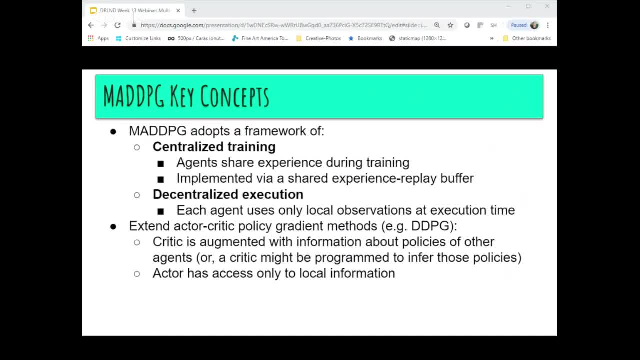 directly. the policies can be shared, or the experience replay buffer can be shared or the critic might be programmed just to infer those policies by by looking at that shared experience replay buffer, but the actor only has access to local information. so you know the two key parts of the gdpg algorithm are are two separate you know parts to begin with and one. 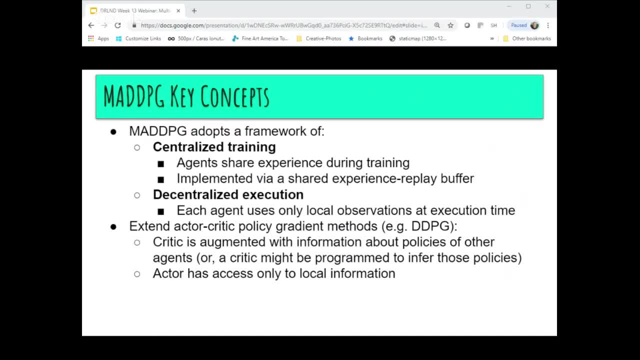 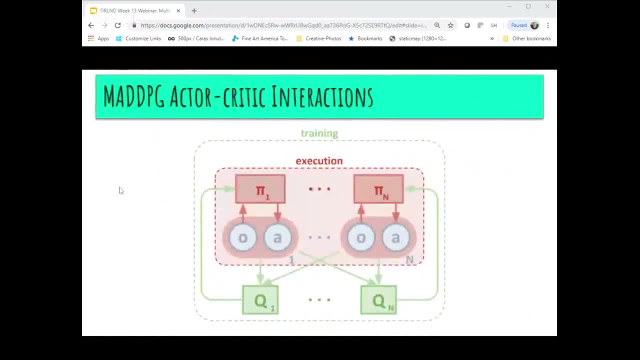 part the critic is is changed. the actor kind of really stays the same as it was implemented in gdpg, with no real change there. this is a diagram from the paper and it just sort of illustrates those concepts. you can see that during training, which is the outer green area, there's a, the, the. 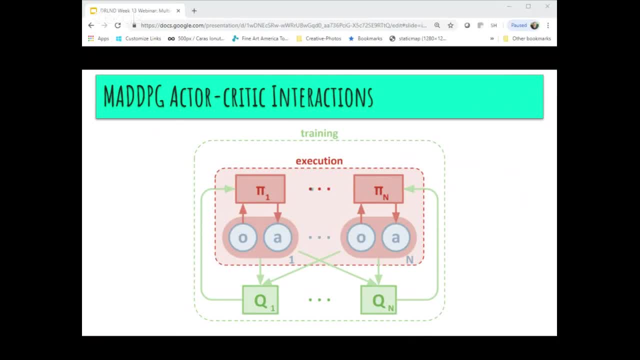 actors in the in the red area. yeah, let's start with that. i guess, uh, the actors are developing and learning a policy based on an offset of observations, they're choosing actions and uh, during training, uh that information, you know is, is fed into the critic network to come up with the q value, to estimate a q value, but also 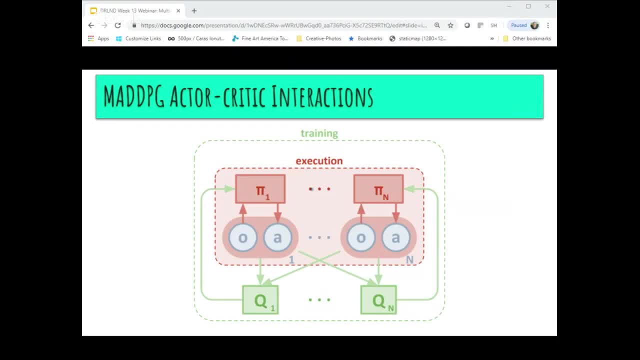 here you can see that there's multiple actors and during training, all those, all that information from all the actors is fed into each and every one of the uh critics, uh, in order to be able to get the information that they need. to get the information that they need to get the. 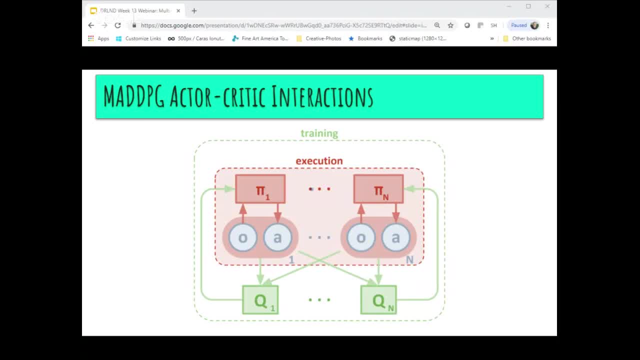 information that they need in order to be able to better understand how these interacting agents impact the environment and be able to get a better estimate of the value of each action is taken as individual states, but then during execution, uh, that green area is, uh is sort of. 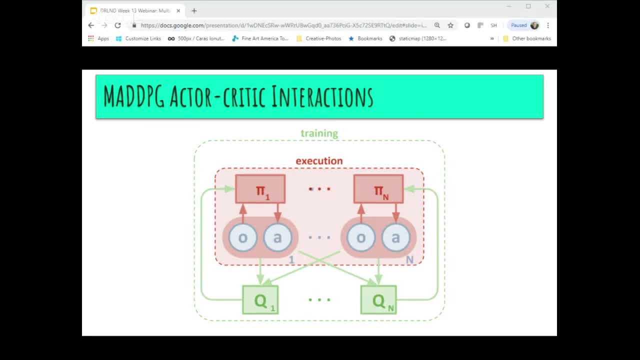 ignored and only the actor uh using local information. uh is used to observe the, the state space and, based on the policy that's been learned, uh choose appropriate actions based just on those observations. so, uh, you know pretty, pretty simple extension related to the ddpg algorithm. so let's talk about some test environments- a good part of the paper. 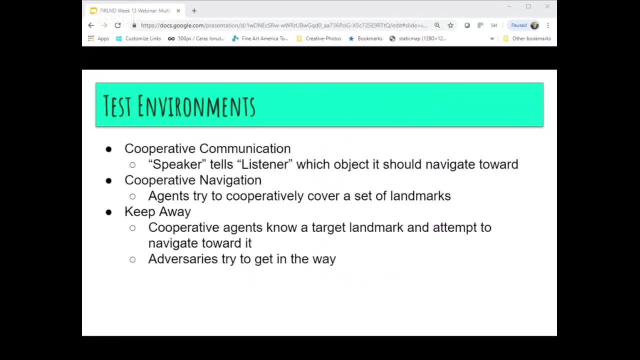 talks about a set of half a dozen or so different environments that they exposed this algorithm to and then compared to the, the baseline ddpg algorithm. and this is just some of those environments. they're kind of interesting in their own right. um, from a individual project kind of perspective, any one of these could have been a. 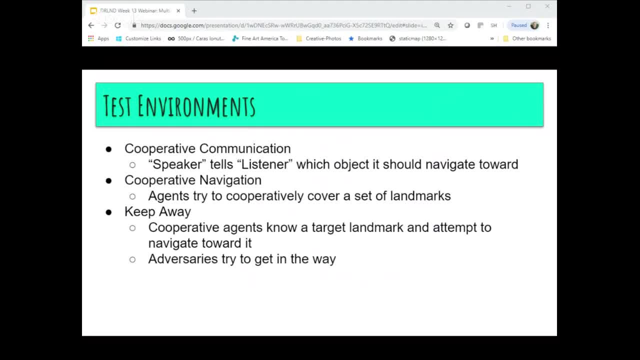 a project to uh experiment with, with uh deep reinforcement learning. so the first these was a cooperative, cooperative communication and in this environment, uh, there's a couple different agents. so one is a speaker, one's a listener and the speaker basically tells the listener which these other objects are, landmarks that are in the environment. 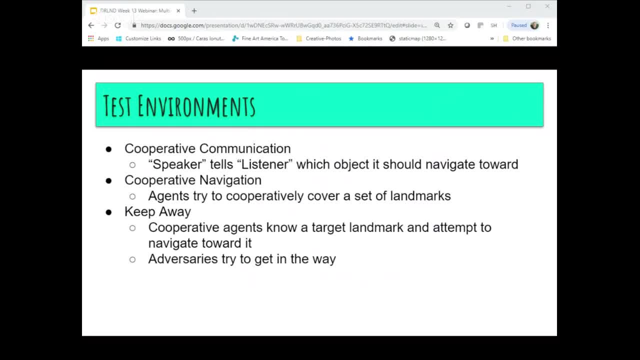 that the listeners should try to navigate towards, and so those are. this is kind of a cooperative uh environment. a second cooperative environment is called cooperative navigation, and in this one uh, there's just a set of cooperating agents and a set of landmarks, and the goal is for uh, all of the agents working together to cover uh all the all the. 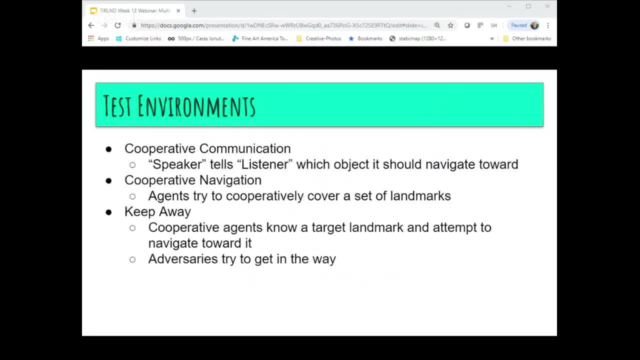 landmarks, and so you know, if they all happen to go to the same landmark there'll be a lot uncovered. they have to kind of cooperate with one another to sort of decide who's going to cover which one, and each move throughout the environment to provide that coverage over the landmarks. then a competitive environment is a keep away. 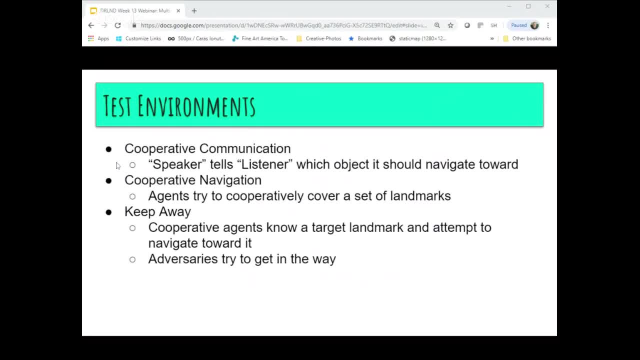 in this one. it's sort of a combination, actually, of competition and cooperation. the cooperative agents- there's a set of them. they all know a target landmark and they all try to navigate towards it. but the adversaries, which are also a number of those agents, they try to get in the way and prevent the, the cooperating agents, from reaching their goals. so 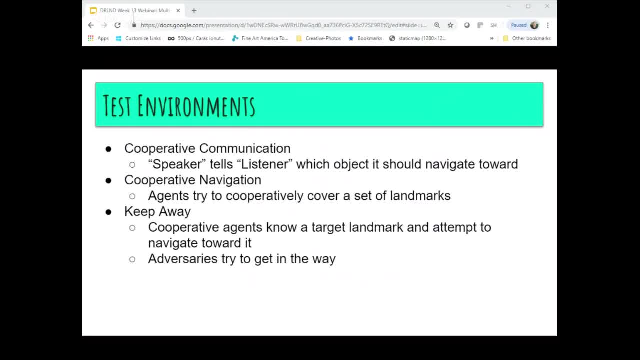 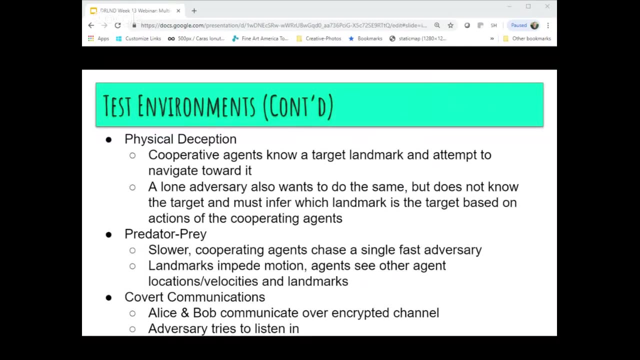 one of them are have a different uh goal in they're trying to optimize for and uh they all you know, are all learning these things at the same time. another environment, physical deception, is sort of again a a combination of cooperation and competition. there's a set of cooperative agents and they know a target landmark and they attempt. 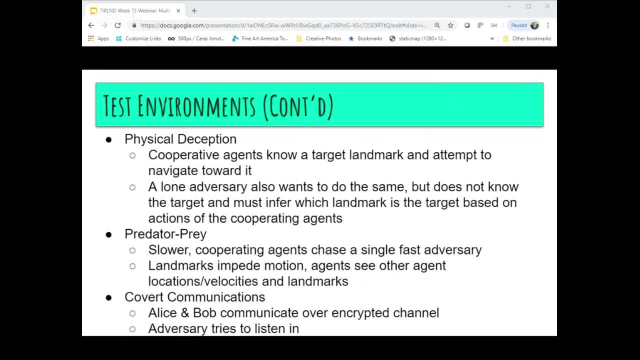 to navigate towards it. at the same time, there's a loan, And the difference is that, while the cooperative agents know which landmark is the target, the adversaries don't, or the adversary doesn't. And so it's called physical deception, because the idea is that the cooperating agents, they somehow have to try to deceive the adversary from inferring which target is the landmark that's the target, one that's supposed to be navigated towards. 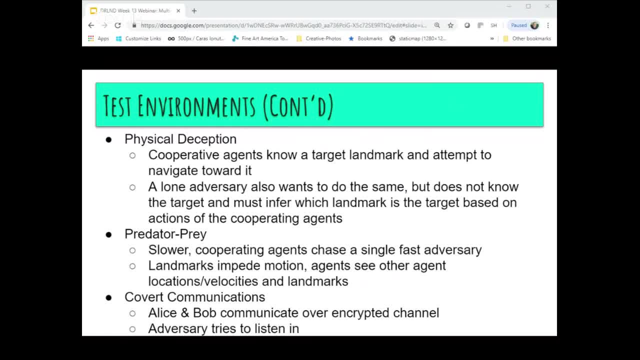 And while they're trying to deceive that adversary, at the same time they're also navigating towards that target. So kind of an interesting environment there. Another truly competitive environment is predator-prey. In this one there's actually a set of cooperating agents. 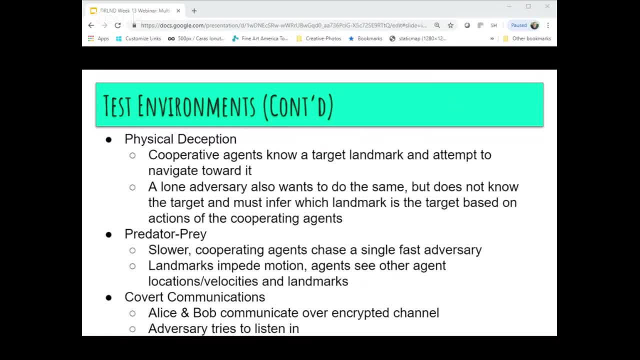 They are relatively slow in moving, and they try to chase a fast adversary. There's a set of landmarks in the environment that impede motion, And so they're trying to chase a fast adversary. And so they're trying to chase a fast adversary. 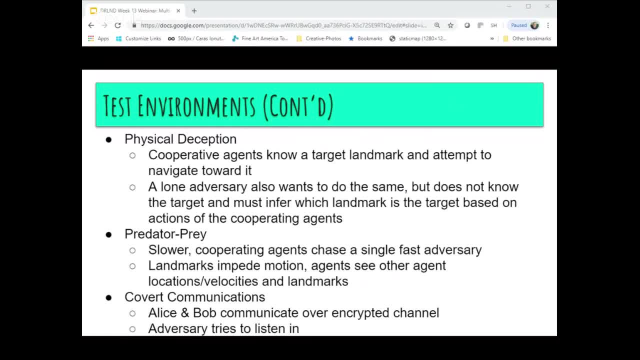 And the agents that are. you know, these slower agents that are trying to face this, trying to track down this adversary. they're given information about the locations and velocities of each other and of the target prey, as well as the location of the landmarks. 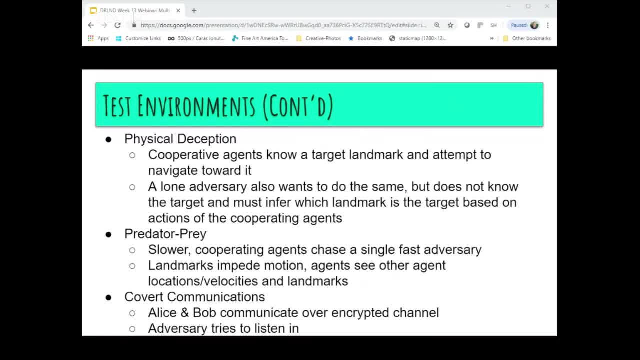 And since the adversary can move quicker, you know he has an advantage, but there's only one of him. So the cooperating agents can, you know, work together to try to pin him down And And actually be able to have one or more of the cooperating agents cover the fast agent, and that, you know, gives them a point in the competition. 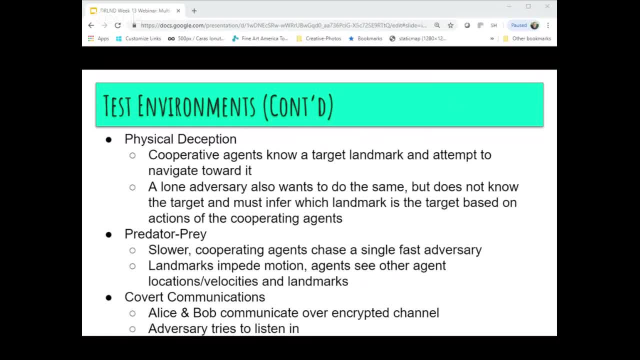 That's a very traditional environment. You see that, not in just deep reinforcement learning, but in you know a lot of different environments, a lot of different methods of trying to solve that particular problem. You see that not in just deep reinforcement learning, but in you know a lot of different methods of trying to solve that particular problem. And so in this you knowρό just going hard and trying to pick the right audience for that task, but it's really straightforward. And so in this you know they're working. really включ everything in trying to make it more seasonal and really solid. And so in this you know, we have bakie with it, And so in this you know them, in this that's, I guess, one boom. they have K différent kind of obviously got That's the taking guy for it. Right, they paid like 50 bucks for essentially a year or so trees together. 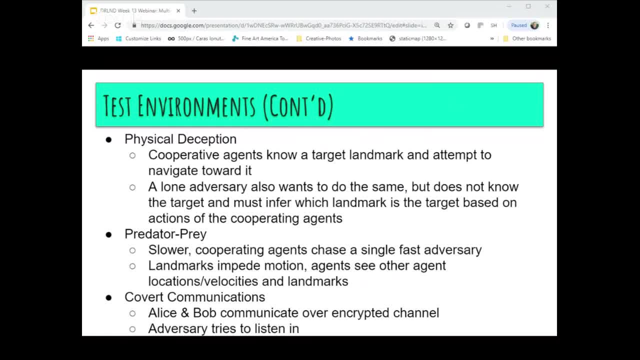 Yeah, Yeah, So, So, So, So, Yeah them them. Um, think about it담, so something else that has live Okay time. So they worked together to try to come up with that communication channel, while the adversaries at the same time trying to learn that same information. 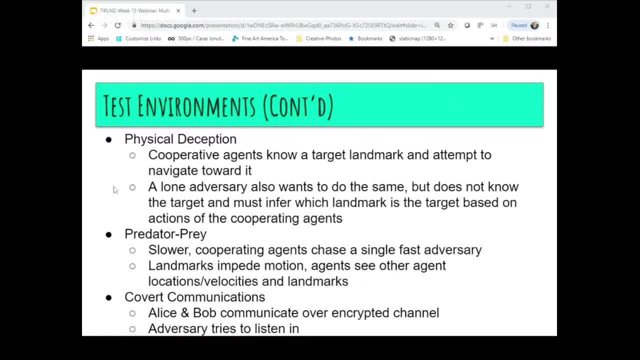 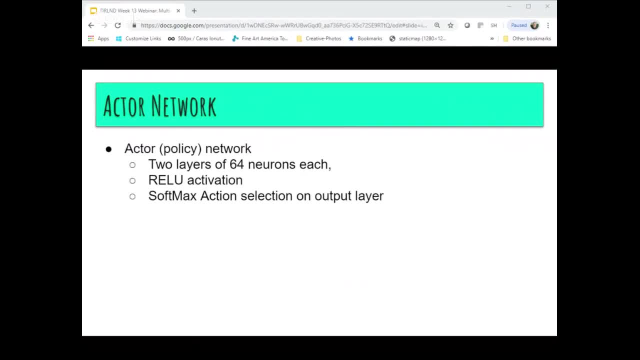 and eavesdrop on their communications. So I might mention I was kind of surprised at how simple the active network was that they used in all these environments. These are to me, I thought, pretty complicated environments And yet, even so, the active network is really a pretty simple neural network. 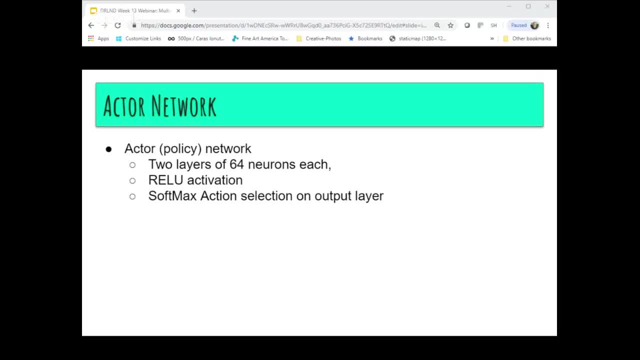 It's a two-layer network, only 64 neurons in each, one simple ReLU activation and then a soft max kind of action selection on the output layer. So a pretty simple neural network And I think you might have found in the first project. 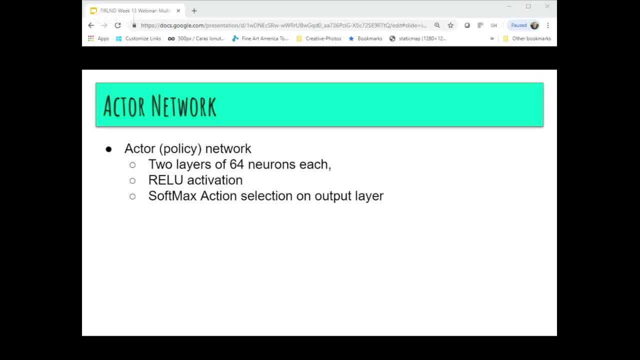 a simple network of 32 or 64 neurons, a couple layers, was actually better at solving that navigation environment than a more complicated network might be. So it's kind of sometimes counterintuitive, It's kind of intuitive of how complex these networks have to be. 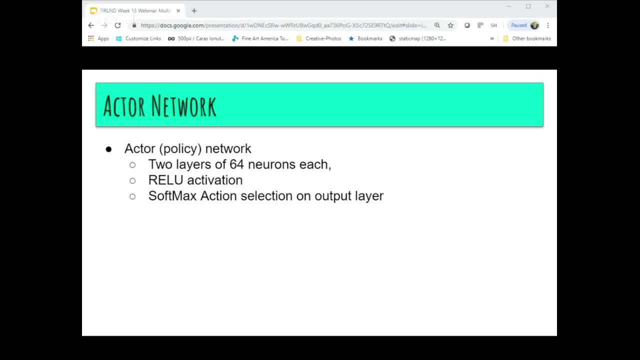 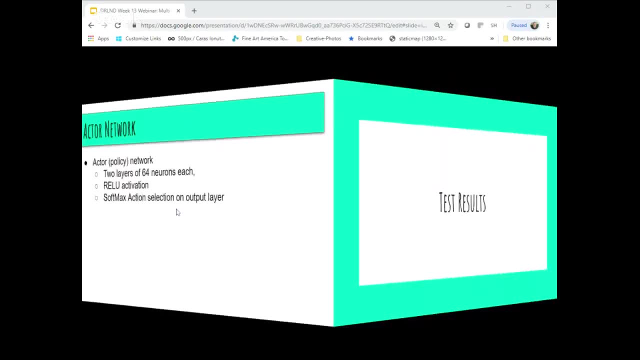 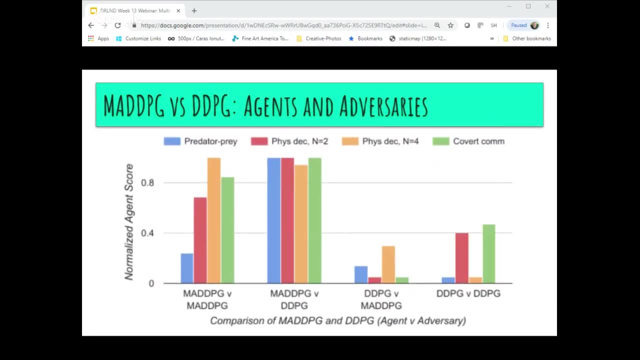 The typical DDPG networks often have 300 to 400 neurons in a layer, So this is a much simpler version of that network. So let's talk about some test results here. I won't go through all the test results. There's quite a few different charts that they present. 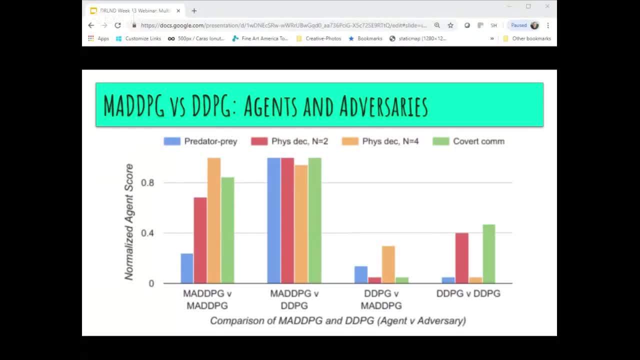 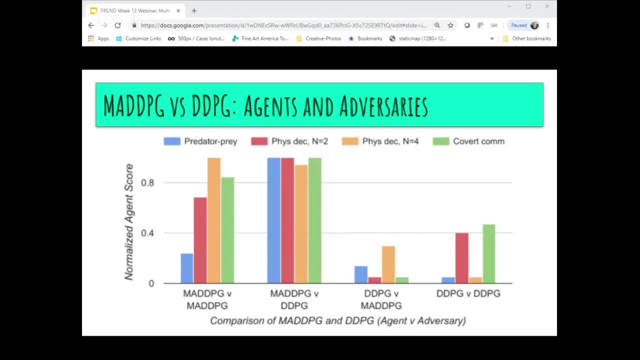 The predator-to-prey physical deception and covert communications. And what this chart kind of shows is they trained agents both with MA multi-agent DDPG and standard DDPG and then kind of compared the performance of the agents against one another. 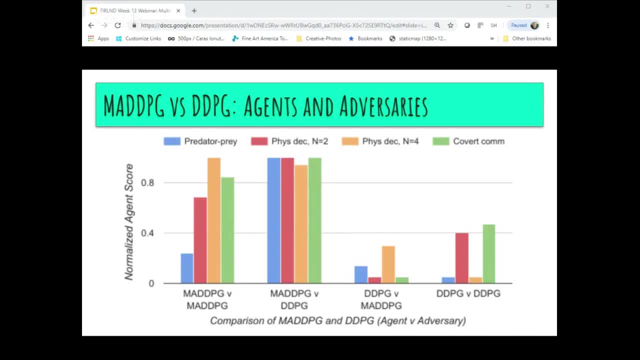 So when both agents were the multi-agent DDPG, both the cooperating and the competitive, the cooperative side of that equation, that's the first set of barges there And you can see that in some of the environments the agent did quite well compared. 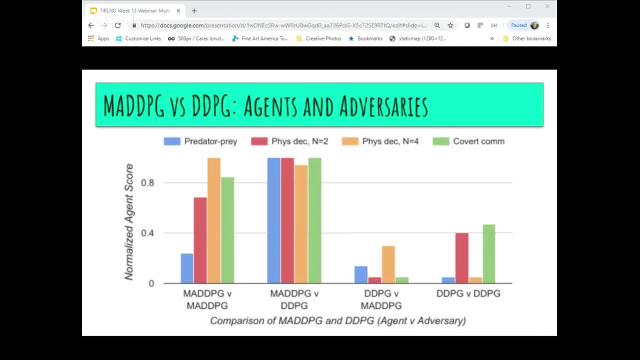 to the adversary, even though they're both using the same algorithm. For example, physical deception with N equal 2 and N equal 4. both did pretty well, as well as covert communications. surprisingly, I think that seems to be one of the more difficult ones, and yet it did pretty well. 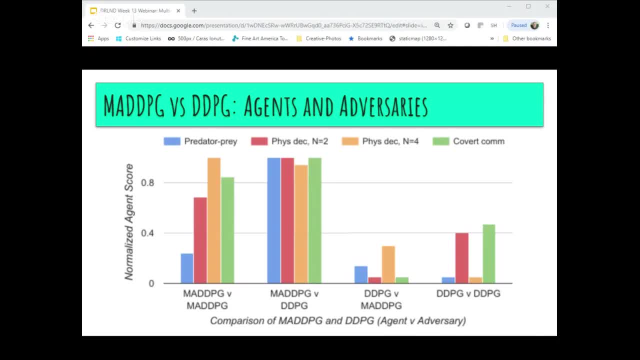 Predator-to-prey not quite as well, Maybe 0.2 agent score, and so it didn't quite do as well in that version when they were both multi-agent. The more interesting one, I think, is the second set there where the agent was programmed with MA DDPG. 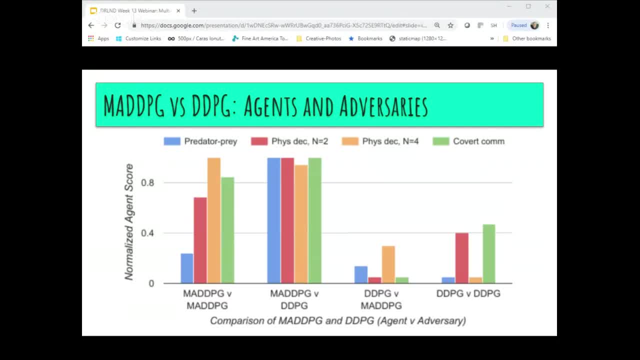 whereas the adversary was traditional DDPG, And you can see that in this case the agent did much better- And that's sort of telling how much better the multi-agent version of the algorithm is than the single-agent version, with scores in around 85% success. 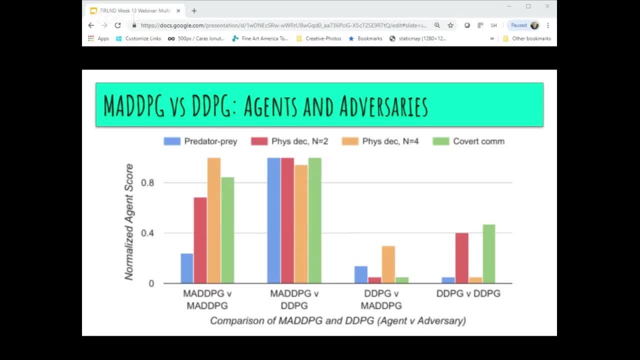 So that's really telling a graphic in that second set. Likewise, the third set is sort of the opposite case of that, where the agent was programmed with the traditional DDPG and the adversary programmed using the multi-agent version, And here you can see that the adversary actually did much better. 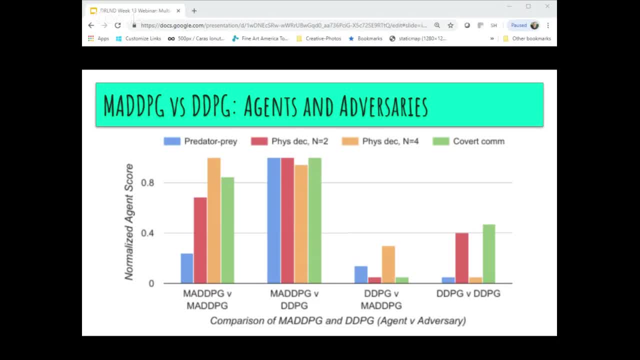 because the agent had a high DDPG, They had a relatively low score. And then you can see the last one just compared both DDPG algorithms for adversary and agent And you can kind of see the troubles that that algorithm just had in general. 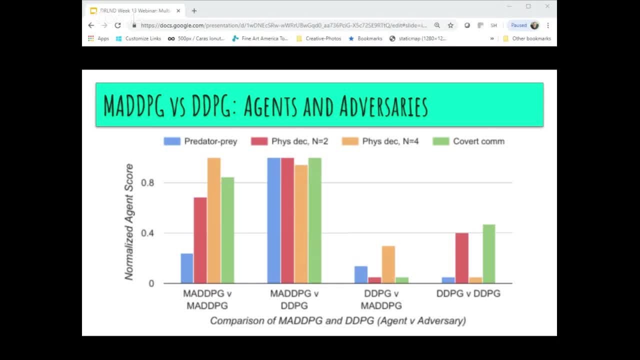 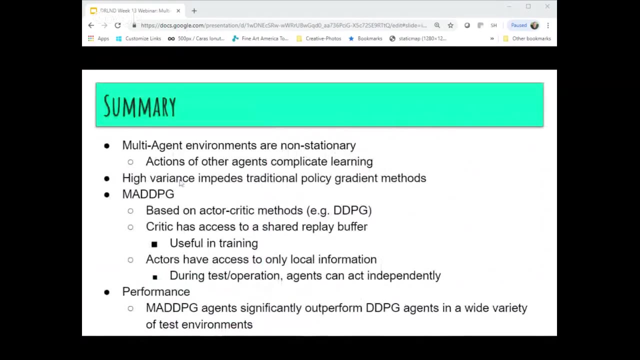 And so the takeaway here is the office kind of showed that the multi-agent version of this algorithm really was a big improvement over the traditional DDPG. So with that, just a summary of today's webinar. we talked about how multi-agent environments are non-stationary and the actions of other agents. they complicate the learning process. 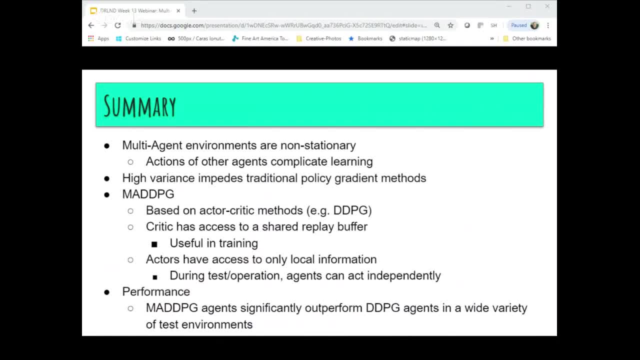 and high variance impedes the policy gradient kind of methods. So the authors of this paper we talked about today, with this multi-agent version- it's based on the DDPG algorithm, the actor-critic standard algorithm- The main change that they made was to have the critic. 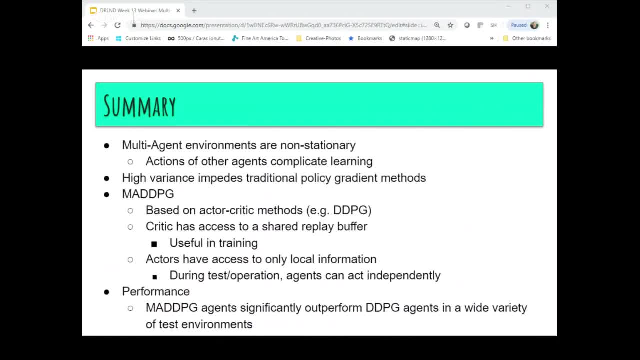 use a shared replay buffer that gives the critic access to the actions and experience of all the other agents that are in the environment. that's used in training, but then, during execution or operation, the actors are used and they only have access to local information so they can act independently one another. 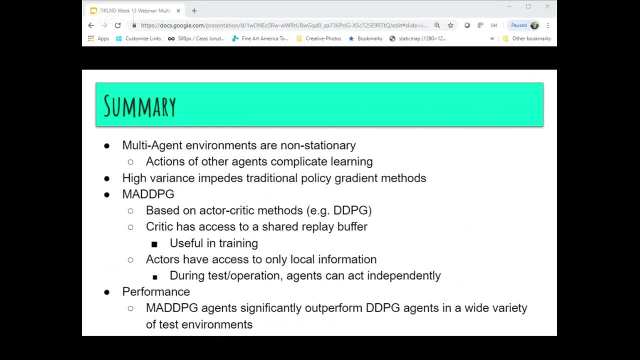 And then we talked about several environments this was demonstrated with- and that's really interesting, We talked about this earlier, So they're both very different- and how the performance of the multi-agent version of ddpg significantly outperformed the traditional ddpg in those, uh, those different test environments. so, um, as i said, uh, it's the. 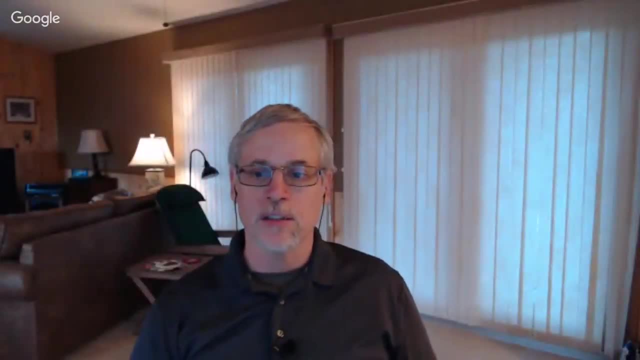 it's a very interesting algorithm. it's a pretty simple extension of the traditional ddpg. i think you'll find in the last programming project for the uh, the deep reinforcement learning nano degree. uh, it's a it's a uh environment where you train two agents that are cooperating with one another.